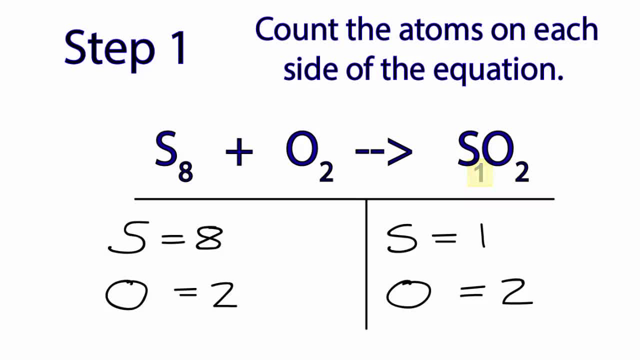 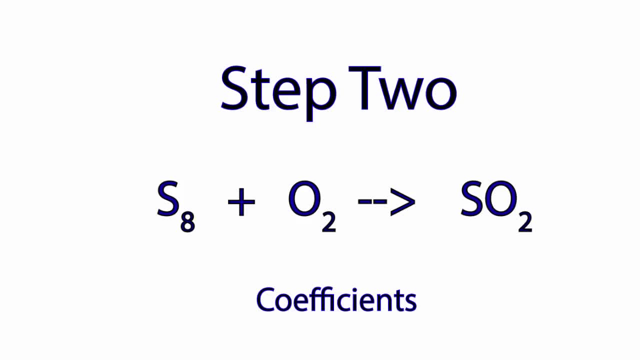 element, we assume that to be one, And that's it. We're done with the first step, Smooth. The big rule for balancing equations is that we can only change the coefficients. Those are the numbers in front of the atoms, The numbers after the atoms, the subscripts cannot be changed. 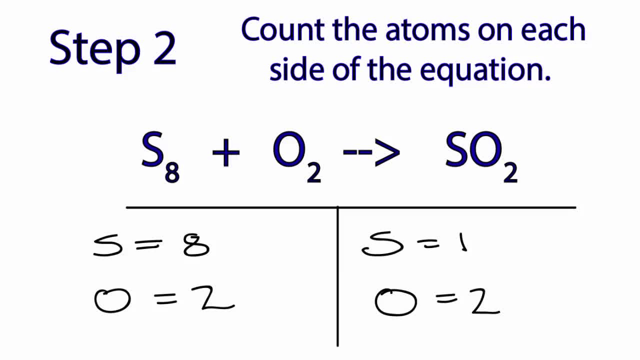 So let's balance this equation by changing the coefficients. If there's no coefficient written, we assume that it's one, So right now there's a one in front of each of these terms. We can see that we have two oxygens on each side of the equation. So the oxygens are fine, But the sulfur. 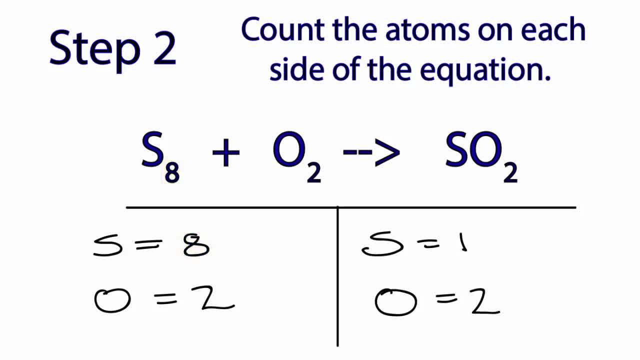 atoms. we have eight on the left side, The reactants, And only one on the right. Well, to fix that, I can change the coefficient in front of the sulfur on the right and make that an eight. So if I put an eight here that means eight times. 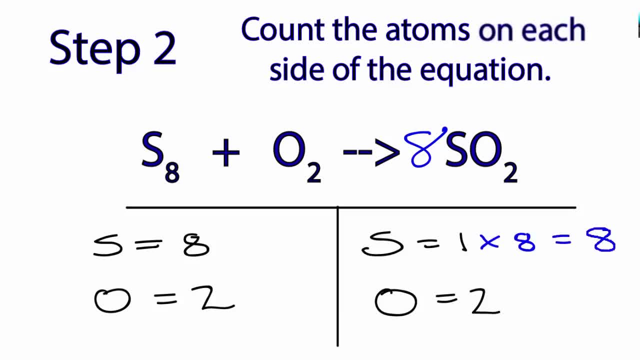 the one sulfur, That'll give me eight sulfurs, And now my sulfurs on both sides are eight. But this eight here is also times the two oxygens And that gives me 16 oxygens. So I've fixed the sulfurs, but the oxygens aren't balanced. 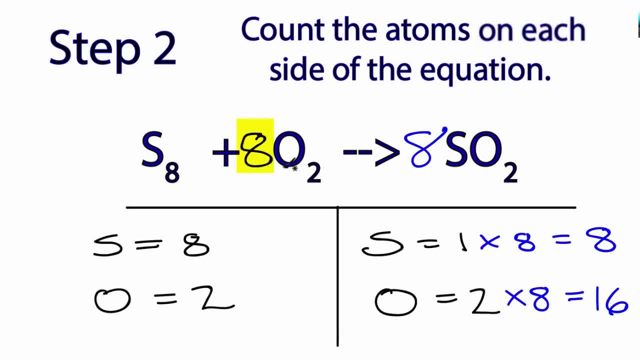 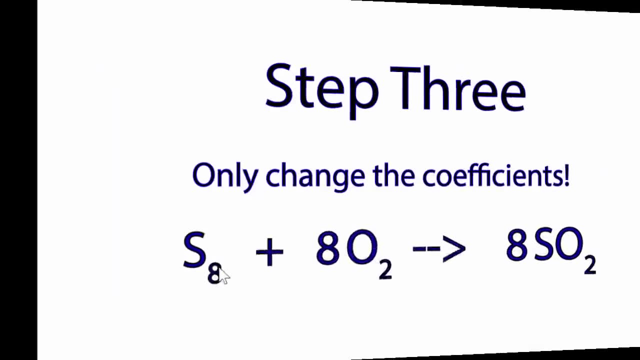 I can change the coefficient here, though, to eight, because eight times two equals 16.. So now I have eight sulfurs on each side, and I have 16 oxygens on each side of the equation. This equation is balanced. Step three: so you don't forget, only change the coefficients. Let's try another problem, So in: 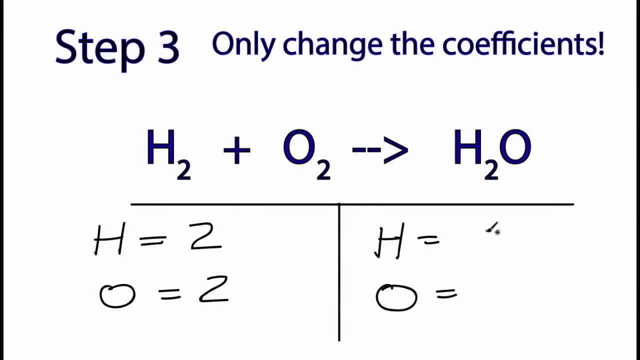 this equation: we have two hydrogens, two oxygens Over here. two hydrogens, One oxygen. How about? let's see, I'll put a two right here. So two times two, that gives me four hydrogens, But two times the one, that'll give me two oxygens. So my oxygens are balanced now. 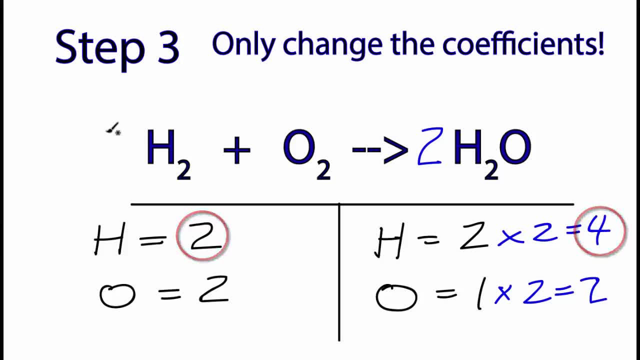 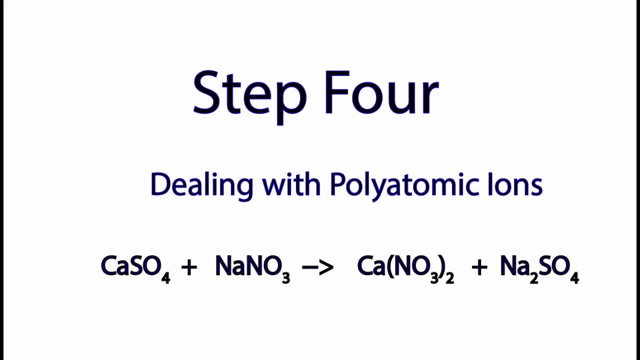 but my hydrogens are messed up. What I can do over here is put a two in front of hydrogen And now two times two. that'll give me four. And now the atoms on each side of the equation are the same. This equation's balanced. Sometimes we'll have equations that look downright scary- Yikes. But if 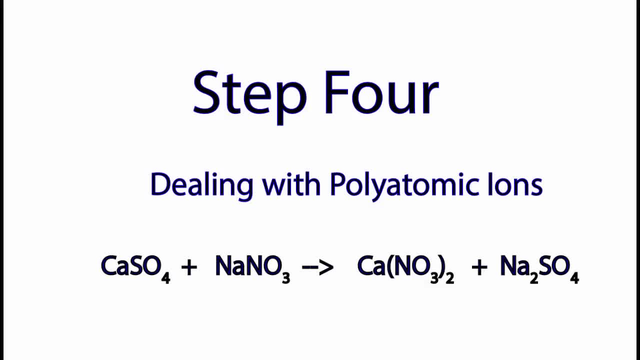 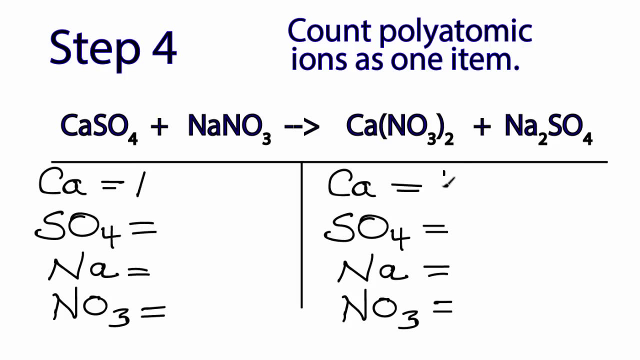 we have a polyatomic ion on both sides, like the SO4 or the NO3, then we can consider that ion to be just one thing. Let's see how that works. So here's the equation and I've done my accounting below. You can see I have one calcium here, one calcium over here, and then I wrote the entire SO4. 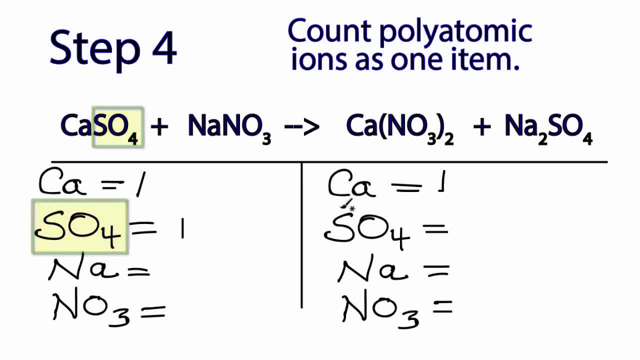 as one thing- And I have one of those here And over here I have one SO4, NAs one, two NAs on this side and over here one NO3. And I have one NO3, but that two on the outside means I have two of them. 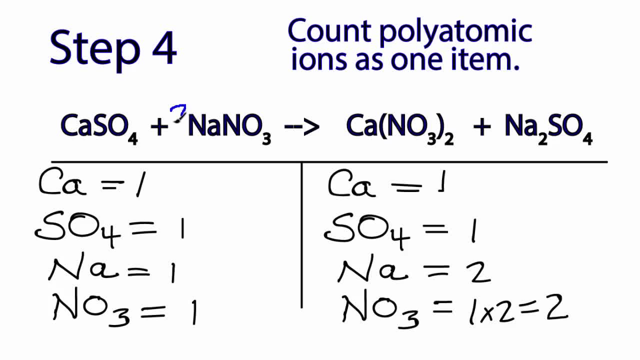 So I have two NO3s. So if I put the coefficient of two right here, that means I'll have one times two two NAs. But this two also multiplies across, So that gives me two, And now everything is balanced. So by treating those polyatomic ions 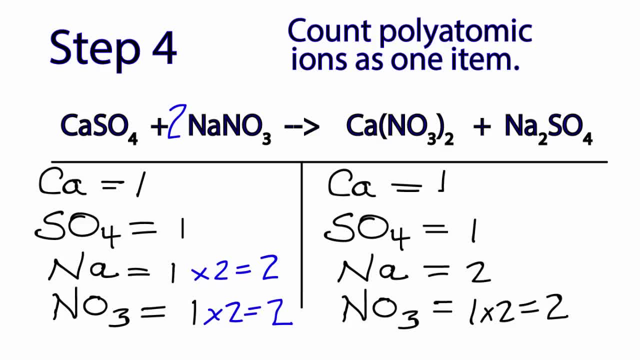 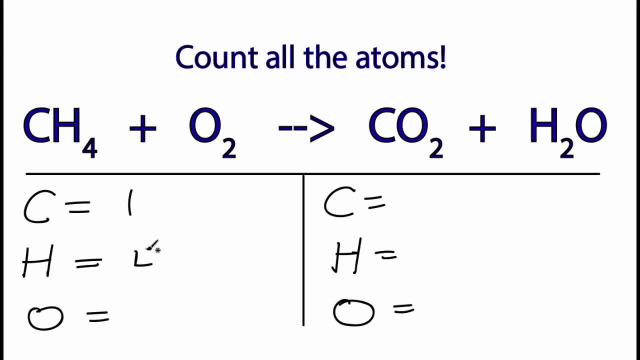 as just one thing. it makes it a pretty simple equation to balance. Let's wrap up with one that sometimes gives people problems. So we can see we have one carbon, four hydrogens and two oxygens. Easy Over here: we have one carbon and then we have two oxygens, and then we have two hydrogens. 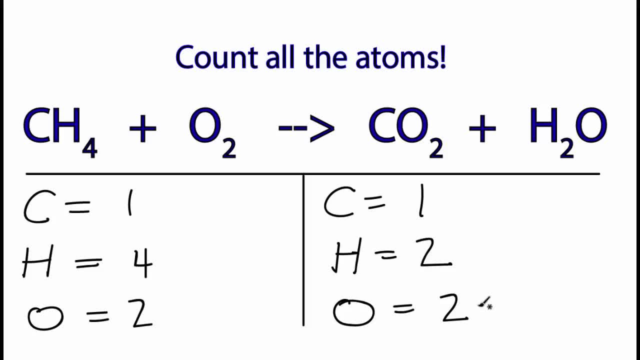 But be careful, We have to count this oxygen over here as well. So we have two plus one. That'll give us three total oxygens. I'll start by balancing the hydrogens. If I put a two in front of this hydrogen, two times two, that'll give me four And that'll fix the hydrogens. But now I have 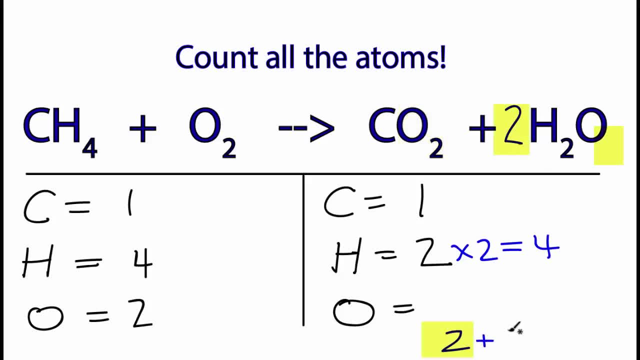 two oxygens plus two times one, two oxygens. That gives me a total of four oxygens. But that's good, because now if I put a two right here and change this coefficient, two times two equals four, and now everything is balanced. 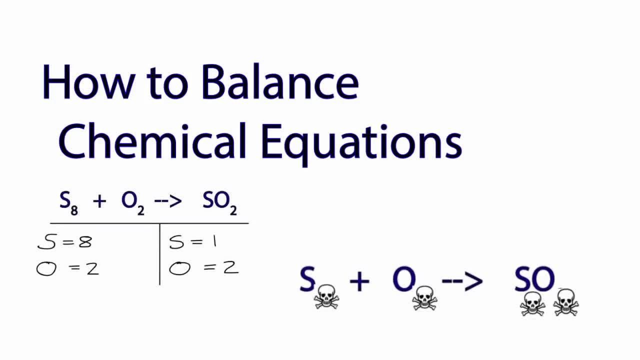 This video has given you the basics for balancing equations, but you've got to practice to gain speed and expertise. The more you practice, the easier it becomes. This is Dr B, and thanks for watching Transcription by CastingWords.